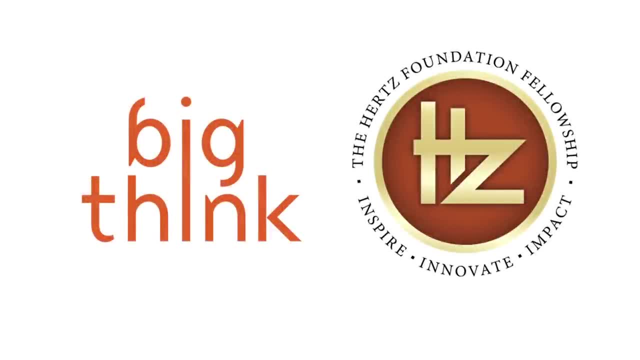 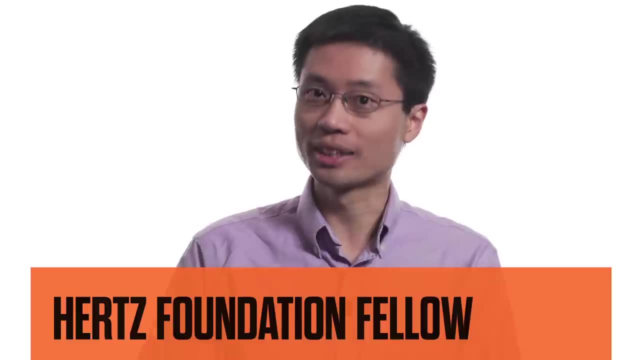 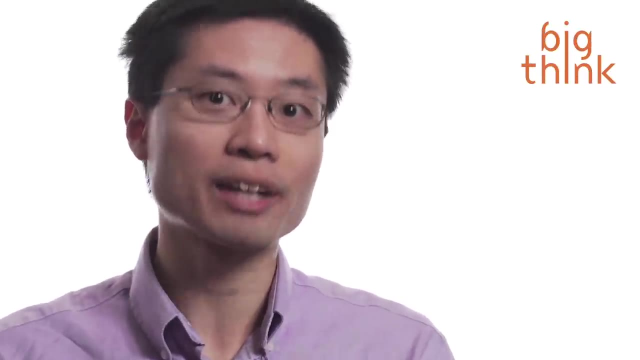 I think that everyone in the world could be a math person if they wanted to. The key word, though, I want to say is if they wanted to. That said, I do think that everyone in America could benefit from having that mathematical background in reasoning, just to help everyone. 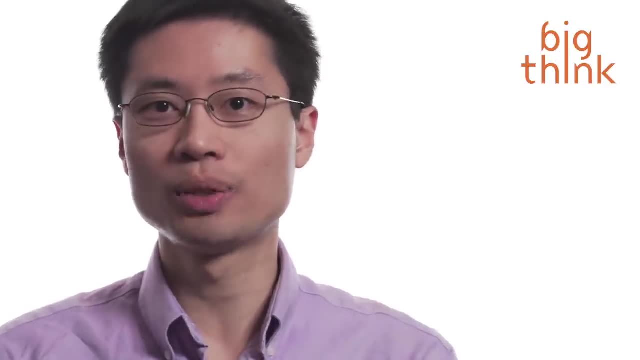 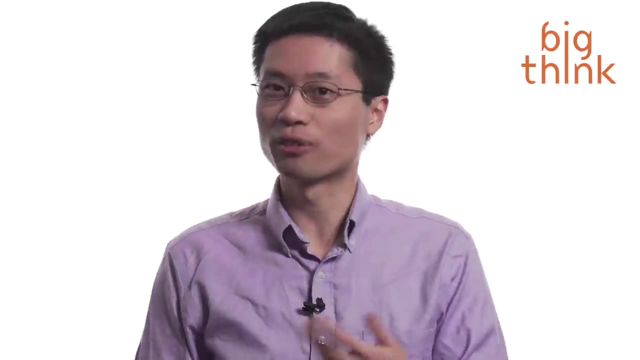 make very good decisions, And here I'm distinguishing already between math as people usually conceive of it, and decision-making and analysis, which is actually what I think math is. So, for example, I don't think that being a math person means that you can recite the formulas. 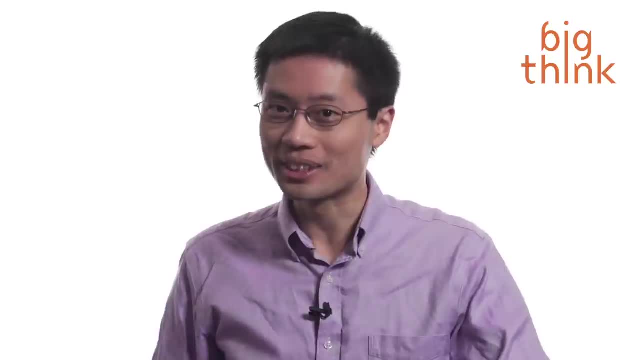 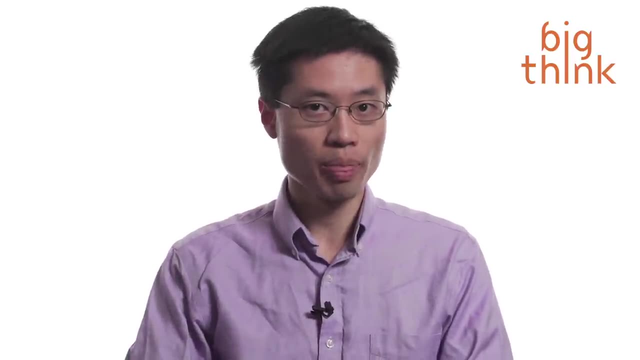 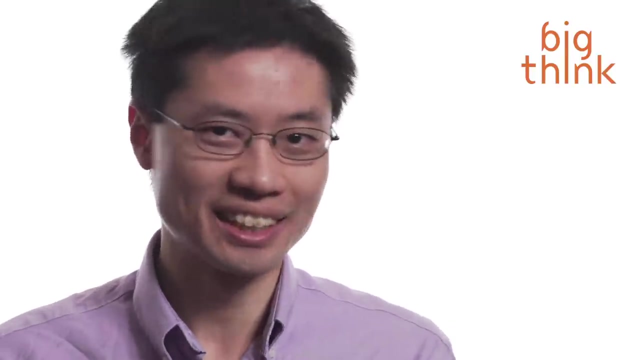 between sines, cosines, tangents, and to use logarithms and exponentials interchangeably. That's not necessarily what I think everyone should try to concentrate to understand. The main things to concentrate to understand are the mathematical principles of reasoning. But let me go back to these sines, cosines and logarithms. 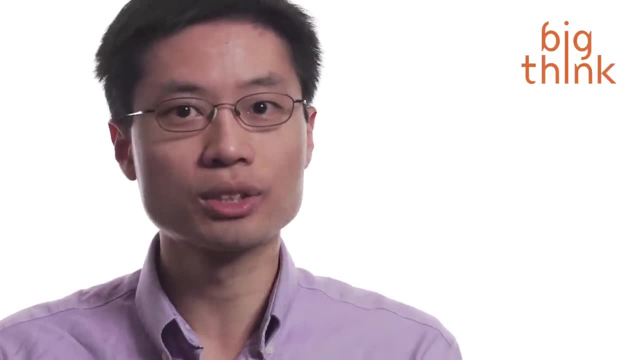 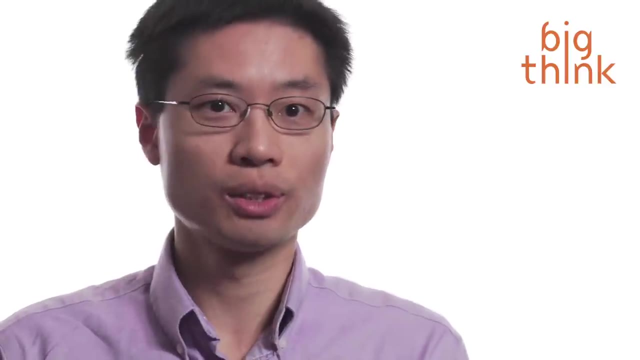 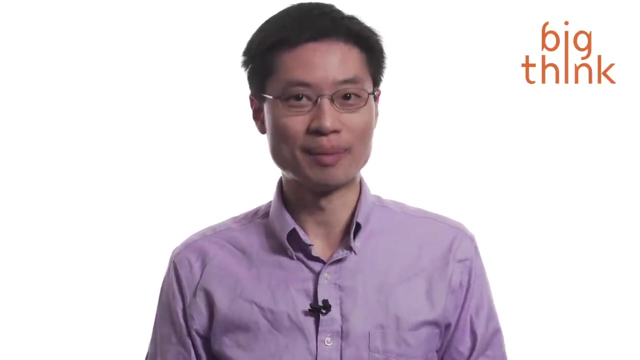 Well, actually they do have value. What they are is that they are ways to show you how these basic building blocks of reasoning can be used to deduce surprising things or difficult things. In some sense, they're like the historical coverages of the triumphs of mathematics. 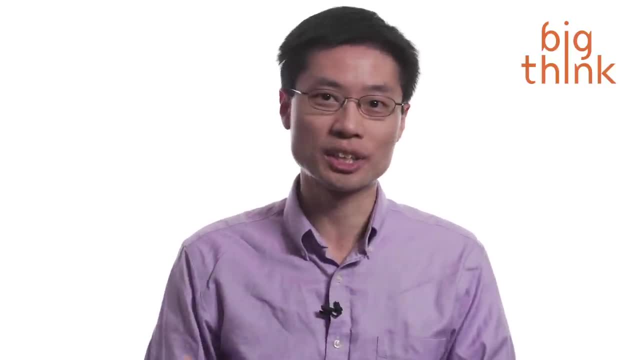 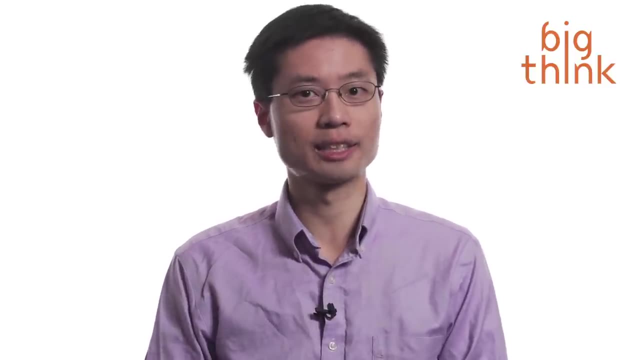 So one cannot just talk abstractly about- yes, let's talk about mathematical logic. It's actually quite useful to have case studies or stories. which are these famous theorems Now? I actually think that these are accessible to everyone. 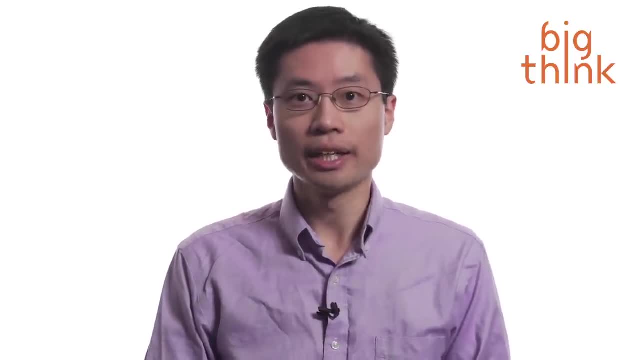 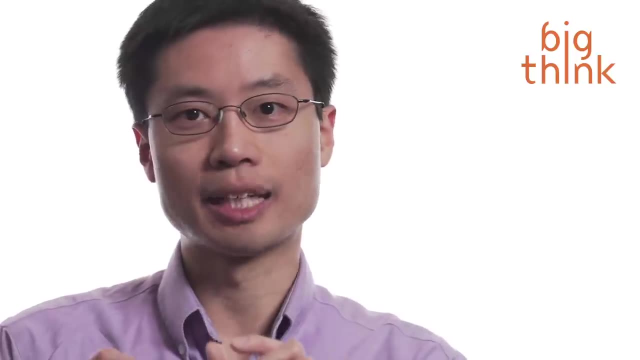 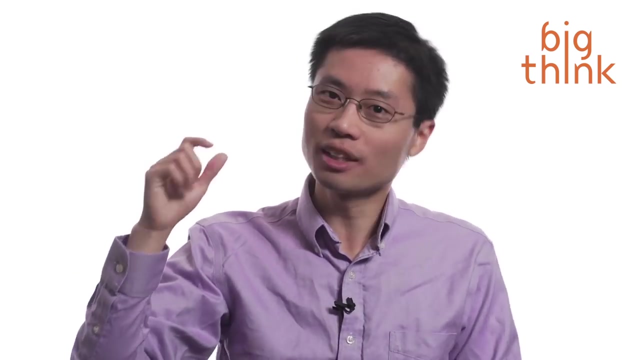 I think that actually, one reason mathematics is difficult to understand is actually because of that network of prerequisites. You see, math is one of these strange subjects for which the concepts are chained in sequences of dependencies. When you have long chains, there are very few starting points, very few things I need to memorize. I don't need to. 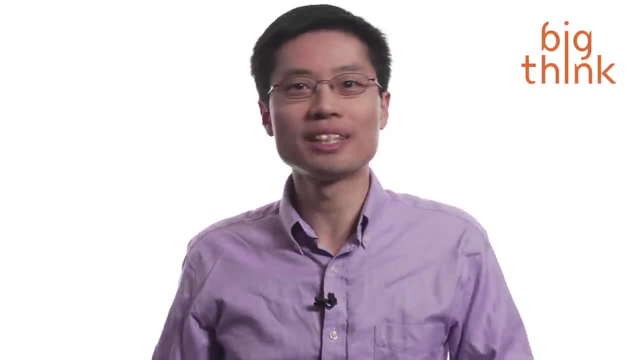 memorize, for example, all these things in history, such as: when was the war of 1812?? Well, actually I know that one, because that's a math fact: It was 1812. But I can't tell. 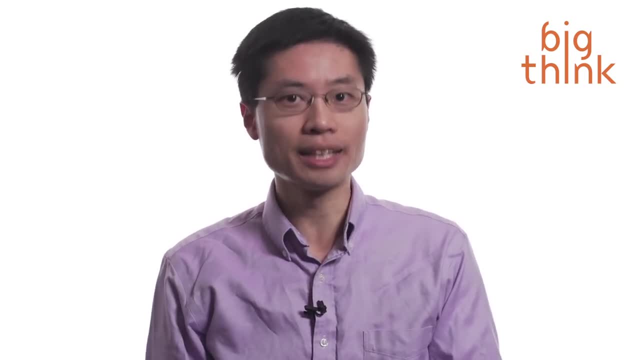 you a lot of other facts which are just pure luck. So I think that there are very few things that are properly memorized In mathematics. you have very few that you memorize and the rest you deduce as you go through. And this: 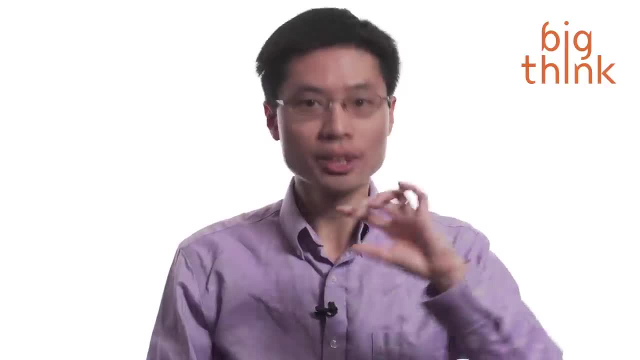 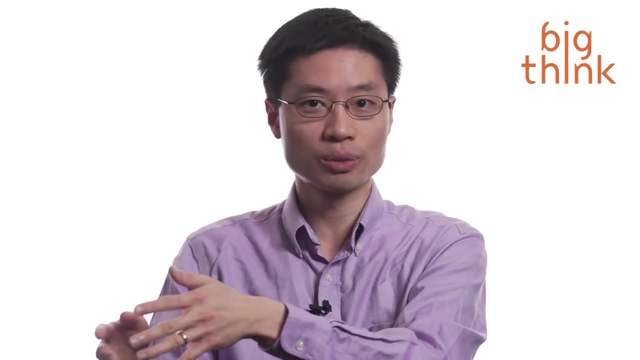 chain of deductions is actually what's critical. Now let me contrast that with other subjects like, say, history. History doesn't have this long chain. In fact, if you fully understand the war of 1812, that's great And it is true. 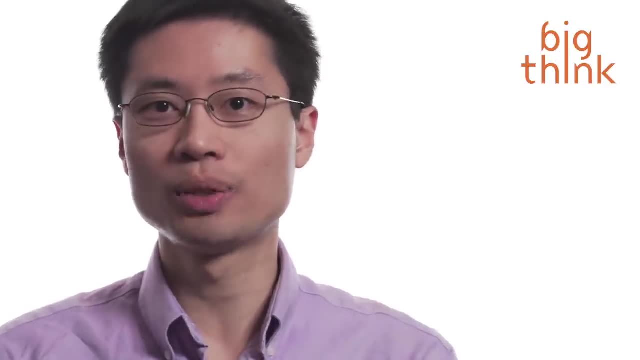 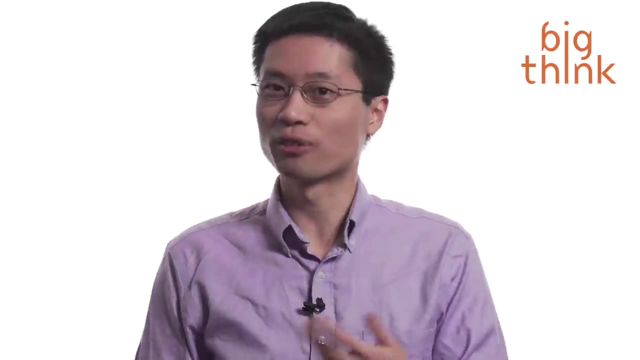 make very good decisions, And here I'm distinguishing already between math as people usually conceive of it, and decision-making and analysis, which is actually what I think math is. So, for example, I don't think that being a math person means that you can recite the formulas. 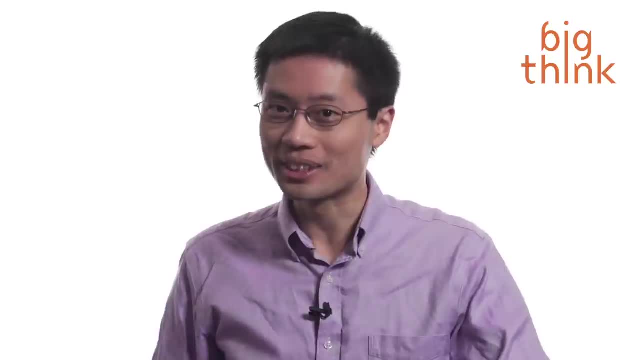 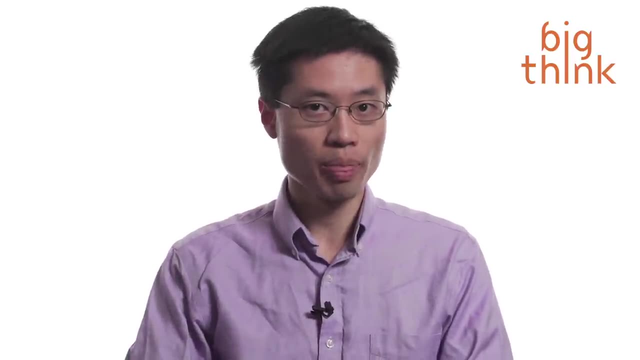 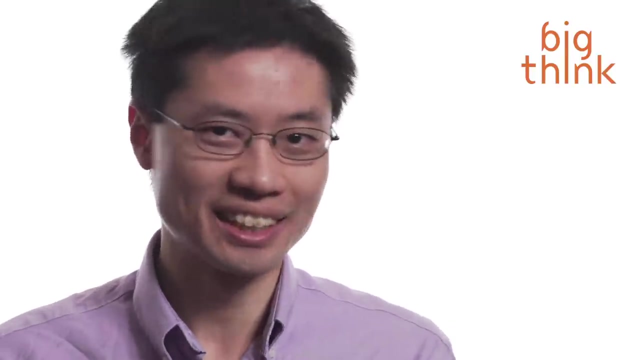 between sines, cosines, tangents, and to use logarithms and exponentials interchangeably. That's not necessarily what I think everyone should try to concentrate to understand. The main things to concentrate to understand are the mathematical principles of reasoning. But let me go back to these sines, cosines and logarithms. 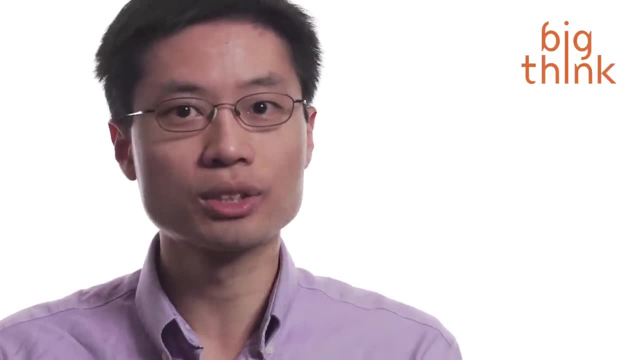 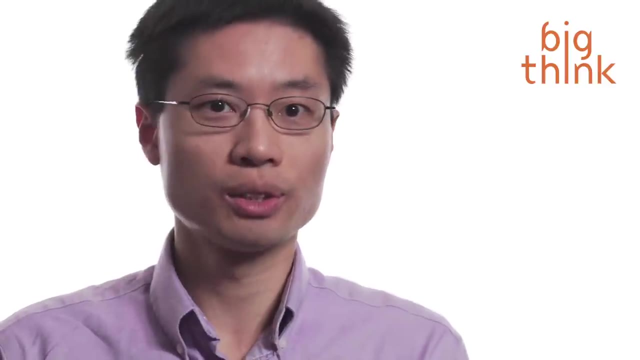 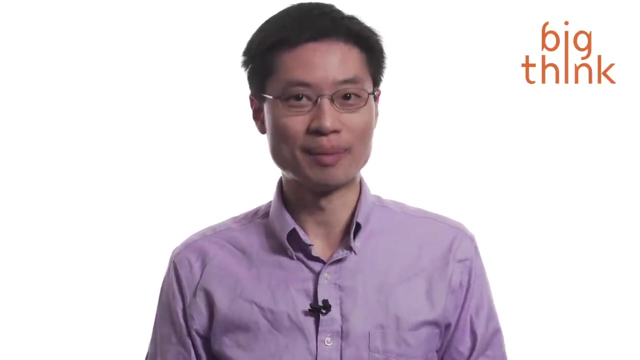 Well, actually they do have value. What they are is that they are ways to show you how these basic building blocks of reasoning can be used to deduce surprising things or difficult things. In some sense, they're like the historical coverages of the triumphs of mathematics. 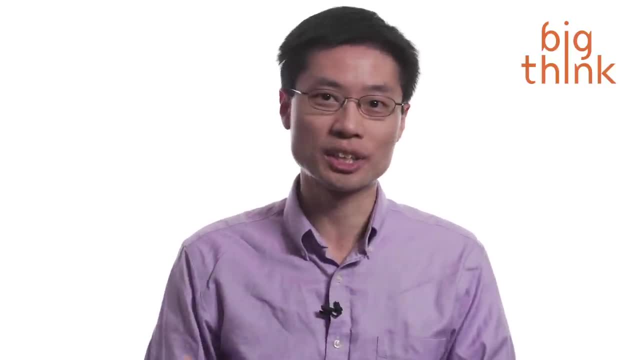 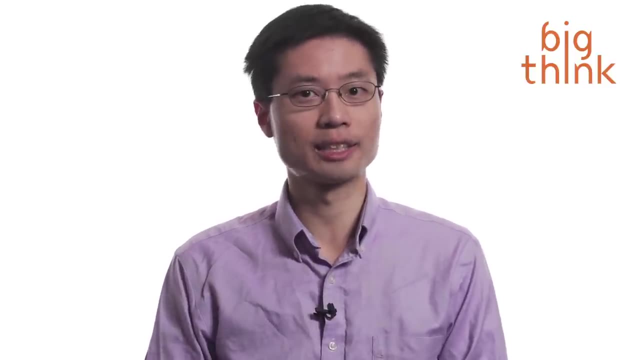 So one cannot just talk abstractly about- yes, let's talk about mathematical logic. It's actually quite useful to have case studies or stories. which are these famous theorems Now? I actually think that these are accessible to everyone. 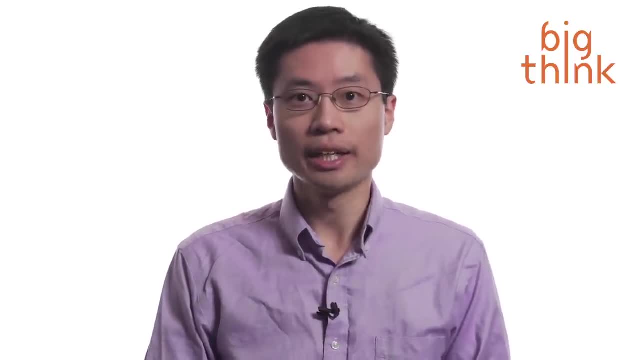 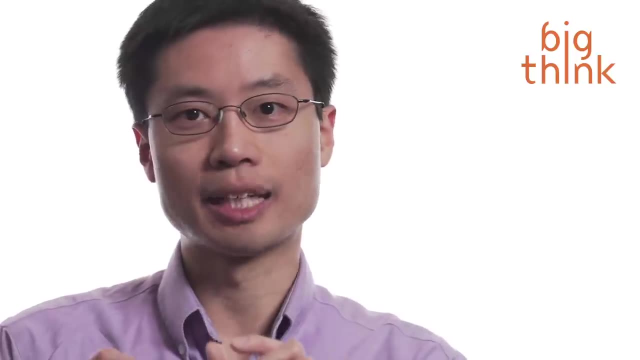 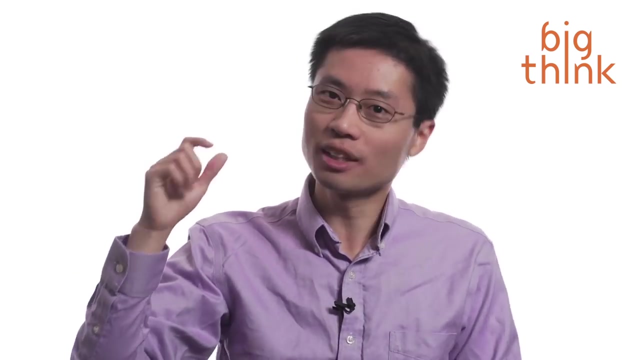 I think that actually, one reason mathematics is difficult to understand is actually because of that network of prerequisites. You see, math is one of these strange subjects for which the concepts are chained in sequences of dependencies. When you have long chains, there are very few starting points, very few things I need to memorize. I don't need to. 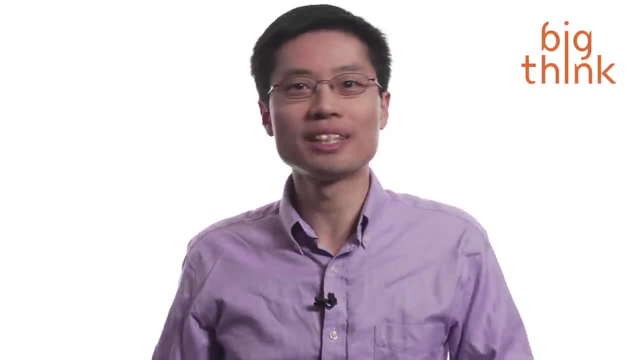 memorize, for example, all these things in history, such as: when was the war of 1812?? Well, actually I know that one, because that's a math fact: It was 1812. But I can't tell. 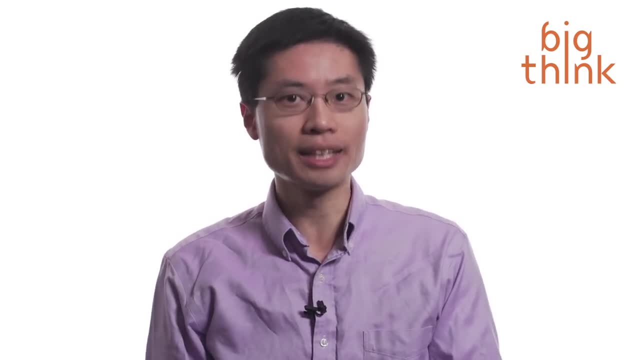 you a lot of other facts which are just pure luck. In fact, there are very few things that are fully memorized In mathematics. you have very few that you memorize and the rest you deduce as you go through. And this chain of 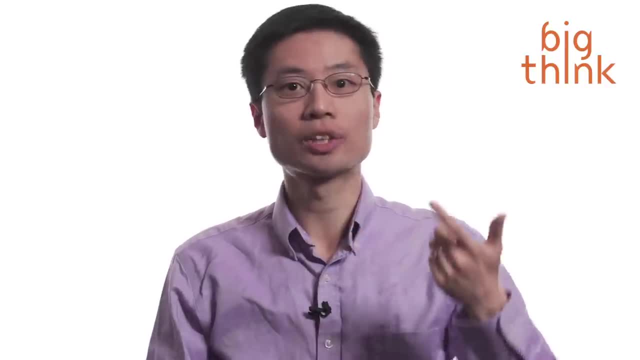 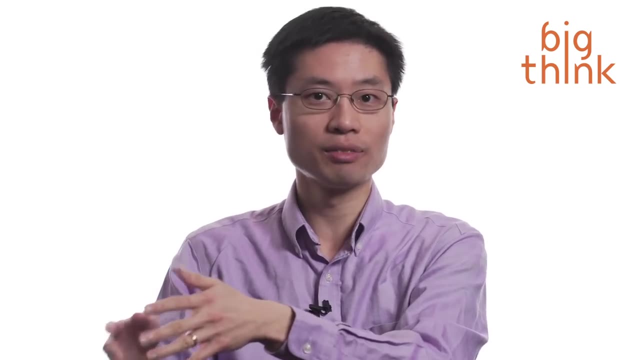 deductions is actually what's critical. Now let me contrast that with other subjects like, say, history. History doesn't have this long chain. In fact, if you fully understand the War of 1812, that's great And it is true. 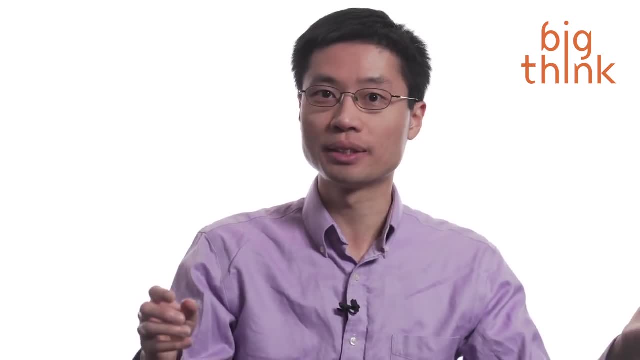 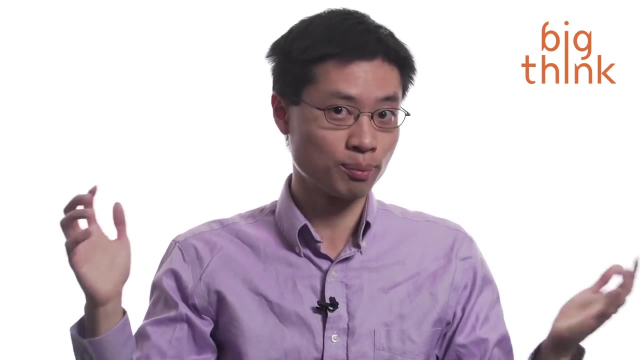 that that will influence perhaps your understanding later of the women's movement, but it won't be as absolutely prerequisite, in the sense that if you think about the concepts, I actually think that history has more than one chain of deductions. The history of the war of 1812 is a chain of deductions And it's a chain of deductions.